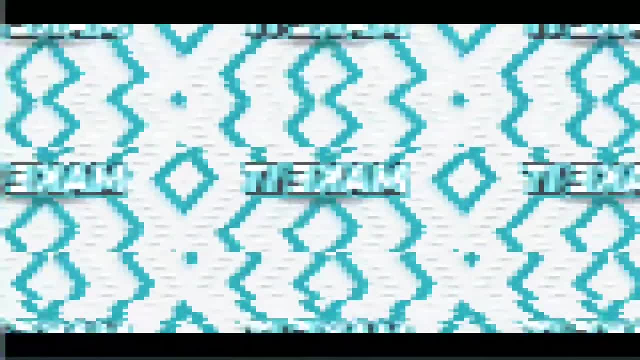 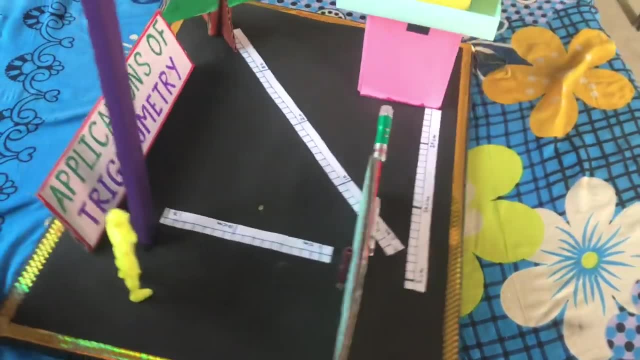 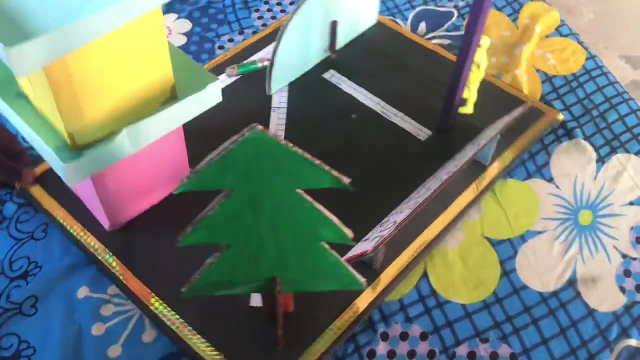 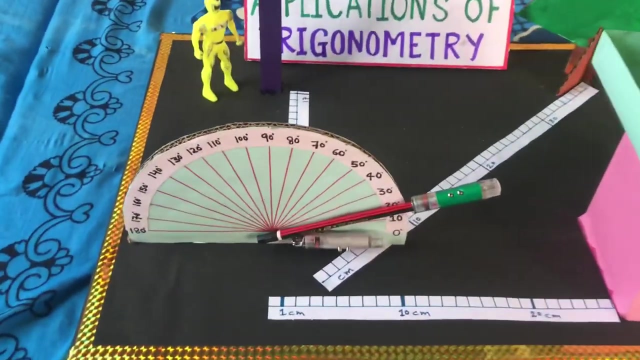 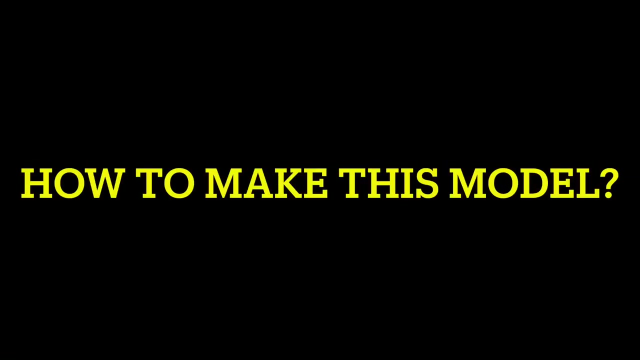 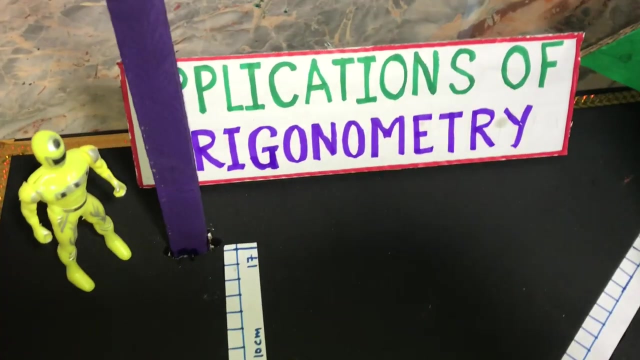 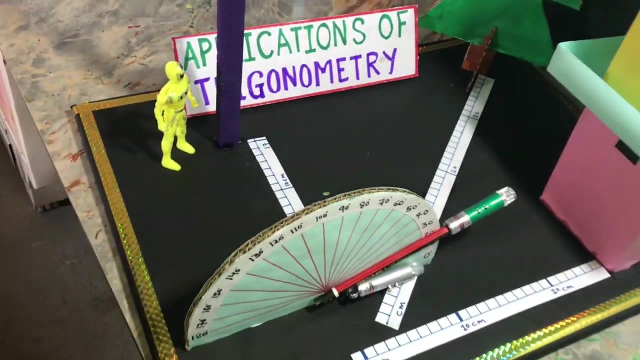 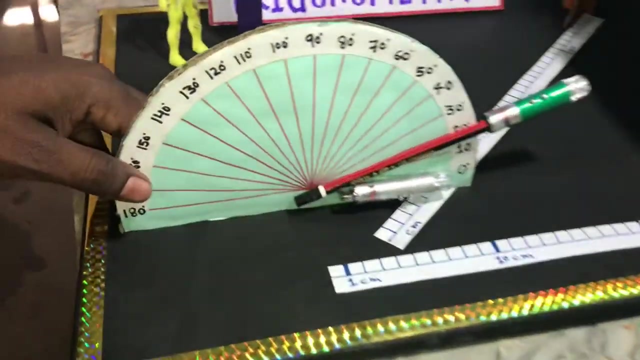 Thank you for watching. Hello friends, this is a mathematical model of applications of trigonometry and it is a working model. Let's see how it works. So the use of this model is that we have to find the height of three things with the help of this clinometer. 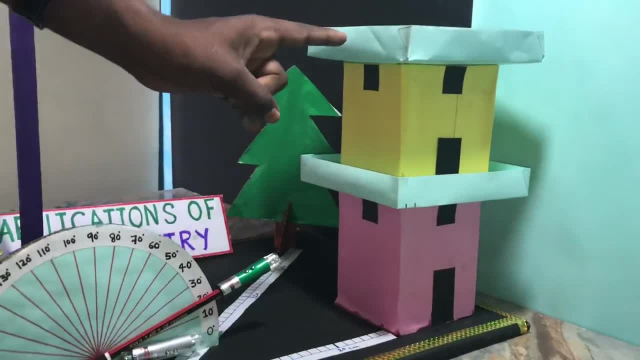 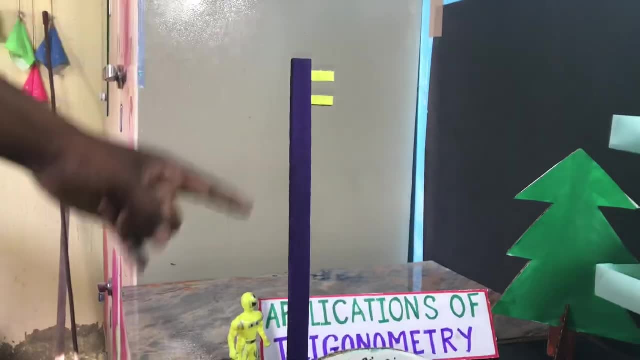 And like this is a building, its height, and then this is the height of the building. We have to find the height of the tree and we have to find the height of a large pole using this clinometer and trigonometry. So this application will be done by trigonometry. 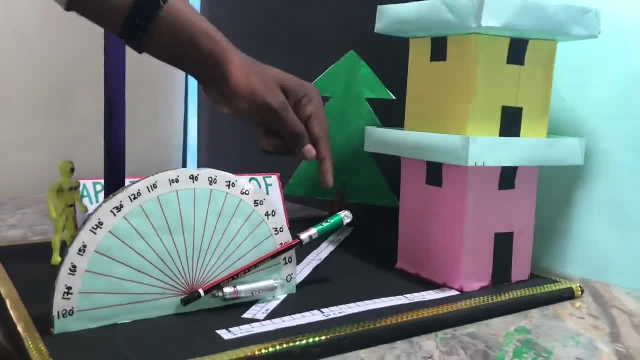 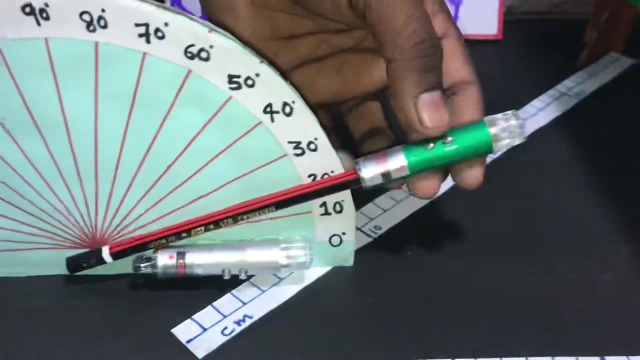 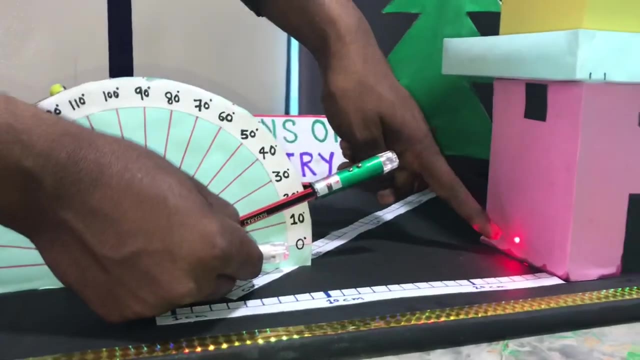 So, first of all, how to find the height of this building. So here I will show you that there is a laser light here, this and this, Because this is the front button. by pressing this it turns on. So see from here, from this angle it is visible. 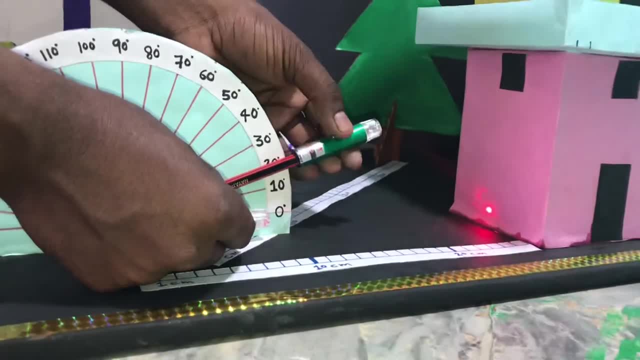 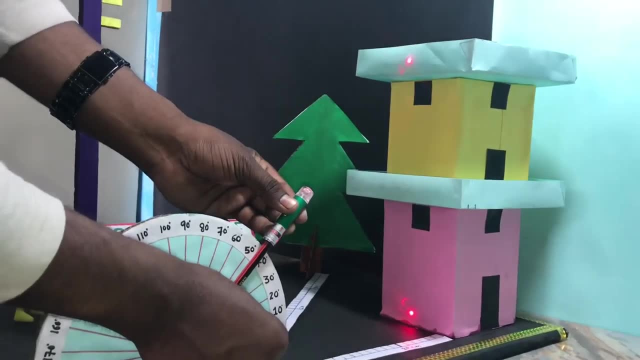 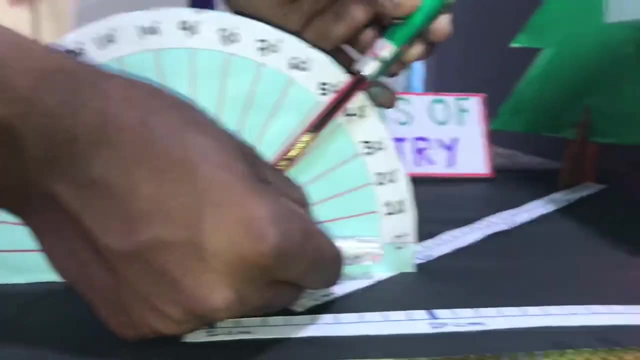 So there will be a slight error of two centimeters. And let's see how much height we have. We are seeing that the angle is 45.. There is an angle of 45 degrees from the bottom to the top, So we will take angle 45.. 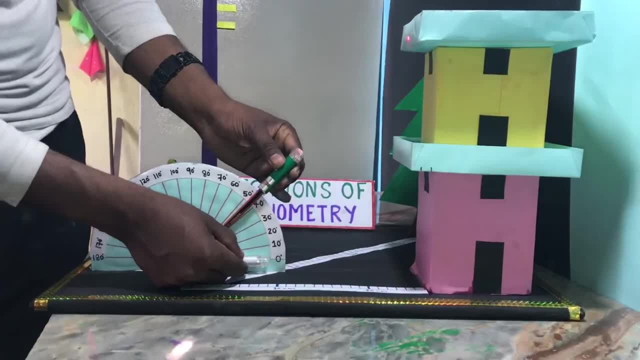 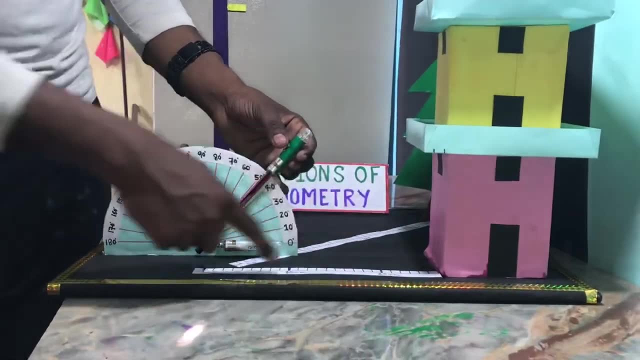 So we can see that a triangle is being made. from here A triangle is being made. This is the hypotenuse, this is the perpendicular and this is the base. So we know the length of the base And here the scale has fit. 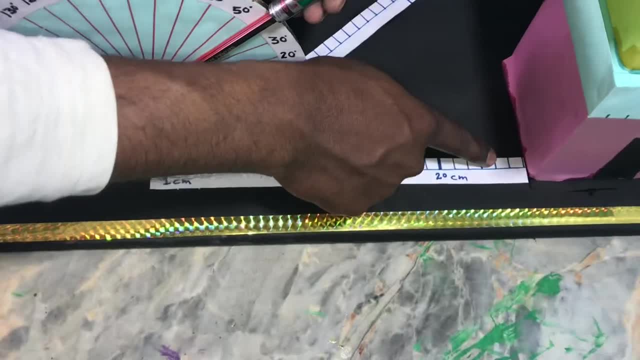 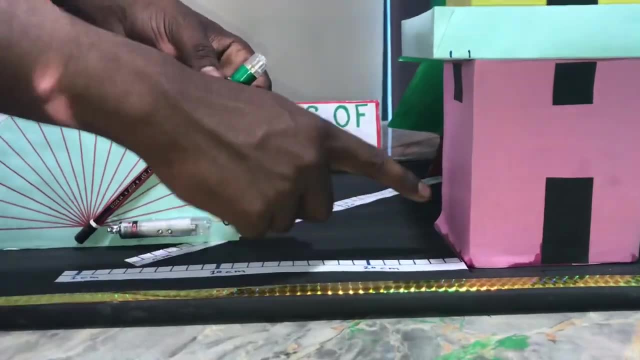 20 centimeters, 21,, 22,, 23,, 24 centimeters, Because this is 2 centimeters, And 21,, 22,, 23,, 24.. 24 centimeters is the length of the base. 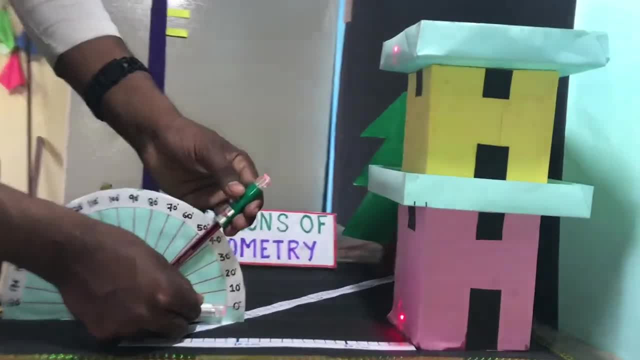 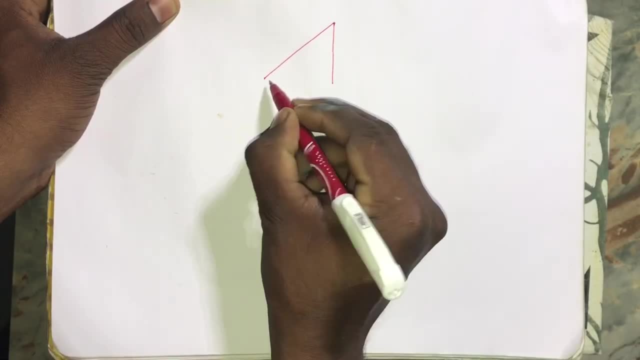 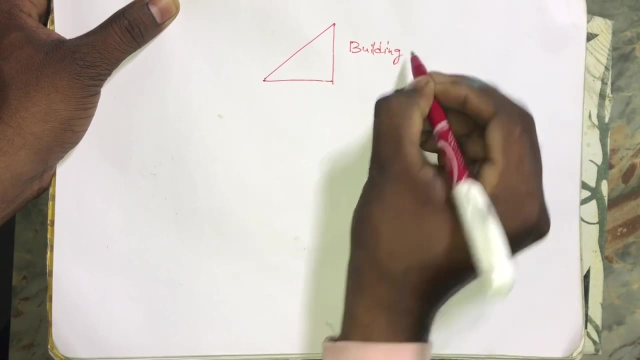 And the angle we have is 45 degrees. So we can find the height of the building by taking 10.45.. This is the height of the building. This is your building And this is your base. This is your hypotenuse. 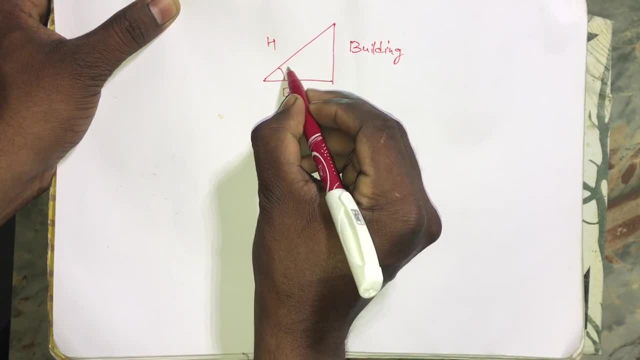 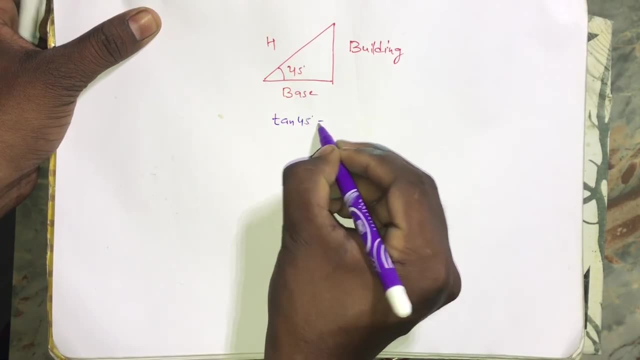 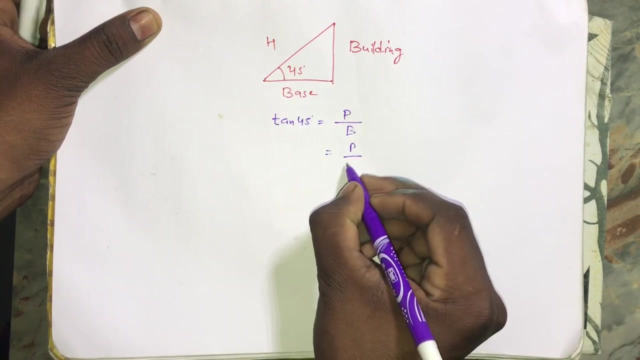 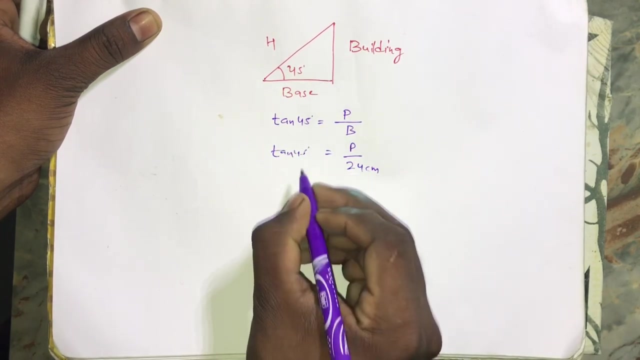 This angle was 45 degrees. 10.45 degrees is equal to perpendicular over base. Perpendicular is unknown And the length of the base is there. Length was there 24 centimeters. We know that 10.45 is equal to 1.. 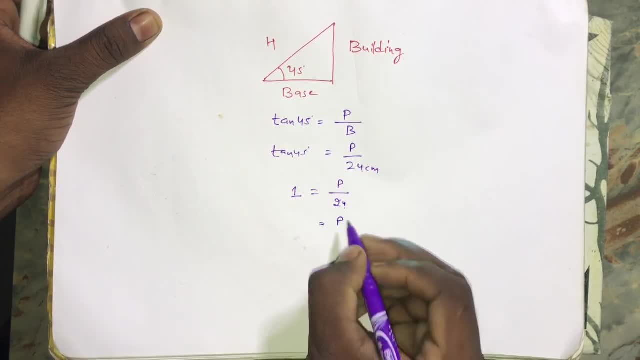 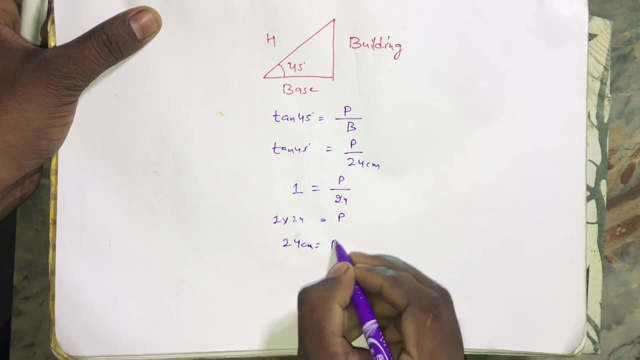 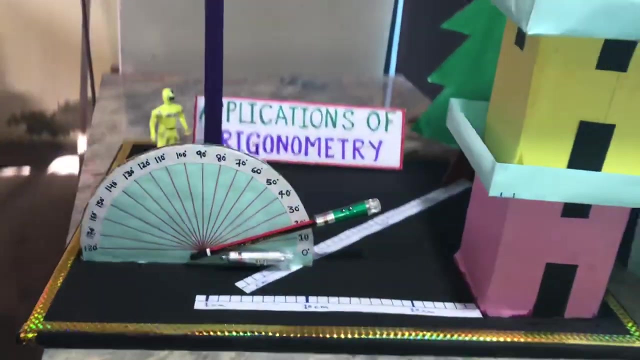 And the perpendicular is here and 24 is here, So the value of the perpendicular will be 1 into 24.. That is 24 centimeters. So this is the height of the building. Next is how to find the height of this tree. 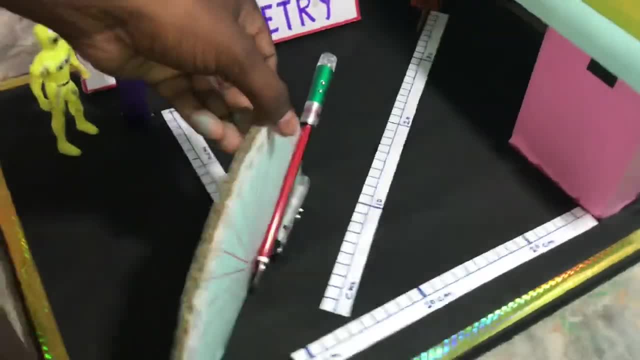 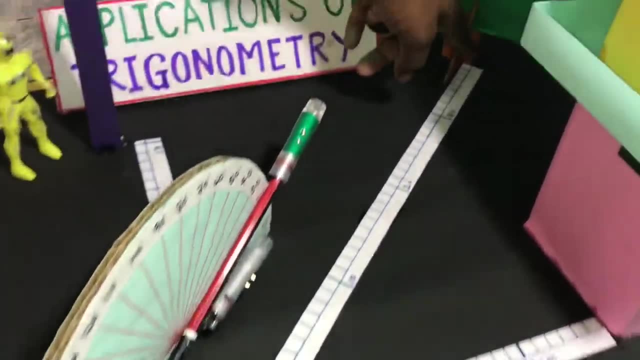 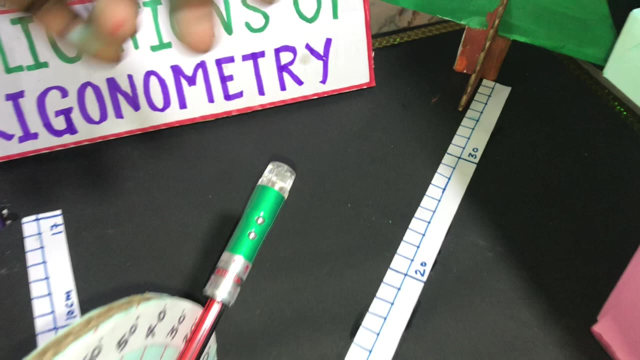 So it bends from here. We will rotate the chronometer And you can see that the length from here to here is 39 centimeters. 39 centimeters. Here we may have a doubt, As we have kept the scale on the base. 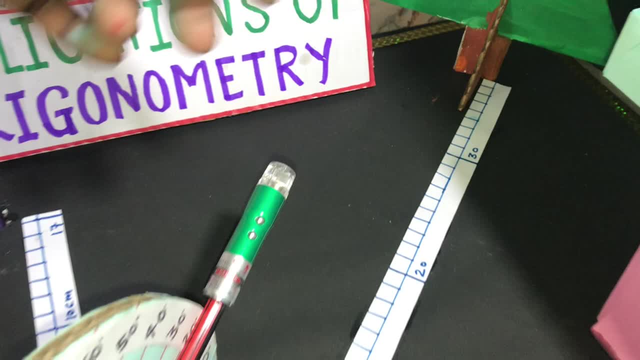 We could have kept it on the tree And the height of the tree had to be found by the scale. But this is not possible in real life. The tree is very long And how will you keep the scale on it? But we can keep the scale easily on the ground. 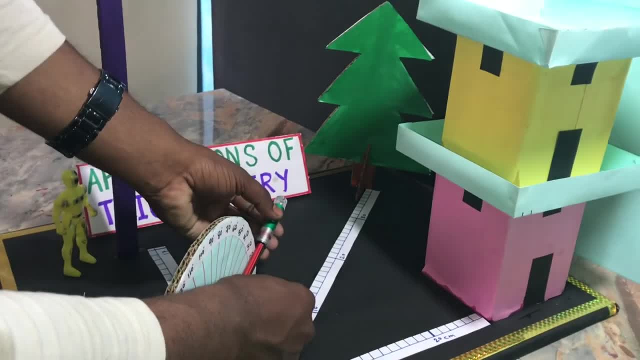 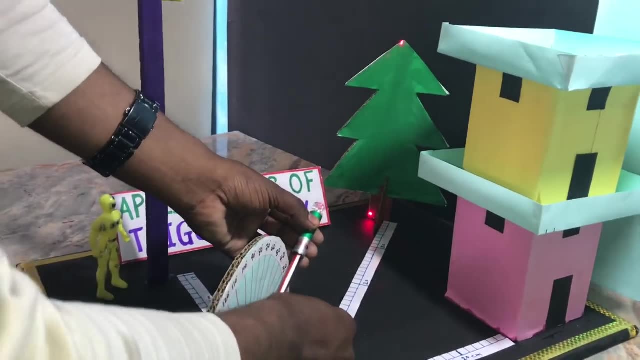 So measure its angle. How many degrees is it? The base starts from here And it ends here, So how many degrees is the angle? The angle is 30 degrees, So from here the formula of 10.30 will be applied. 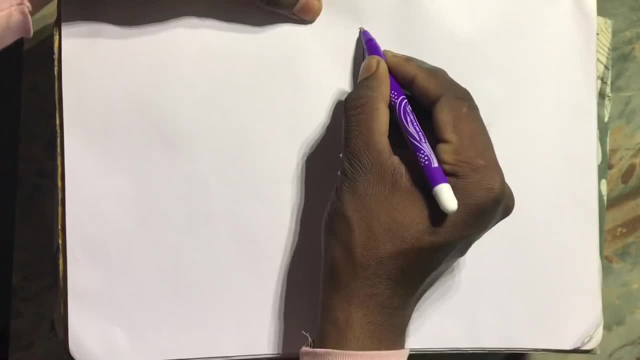 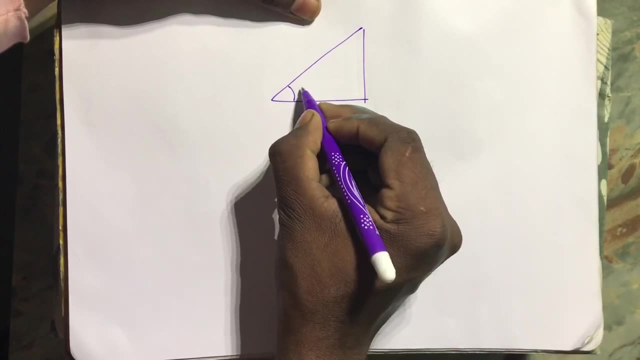 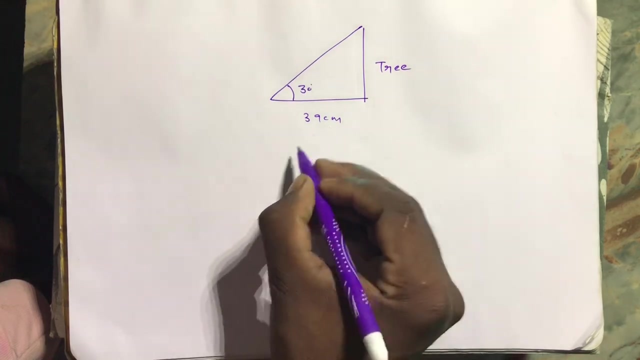 Ok, Let's draw the tree. This was your tree. The tree is 39 centimeters long And the angle was 30 degrees. Ok, So this is the tree. So to find the length of the tree, we will apply: 10.30 degrees is equal to perpendicular over base. 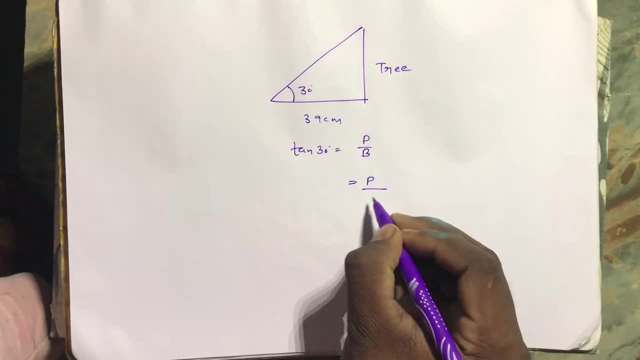 The perpendicular is unknown And the value of the base is 39. And the value of 10.30 is 1 by root 3.. So from here we will cross multiply it- 39 is equal to p into root 3.. 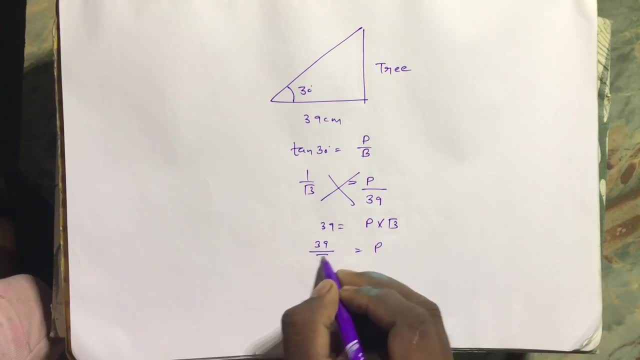 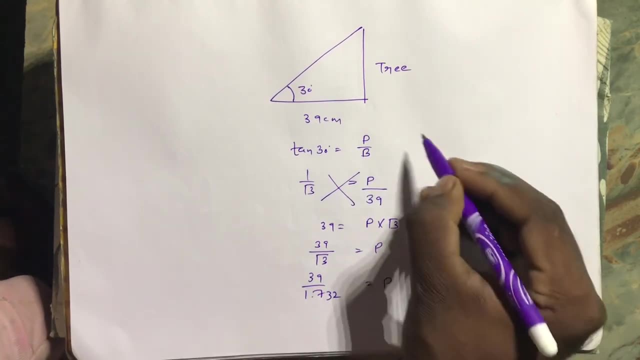 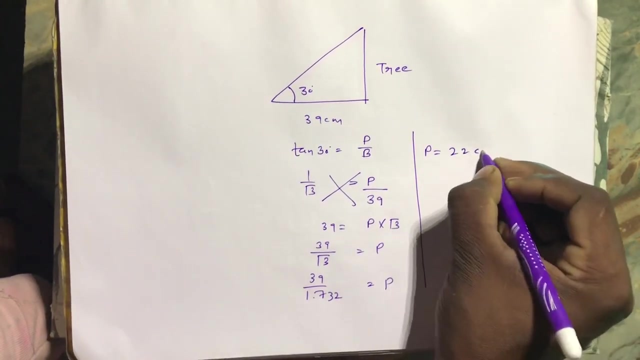 And p is equal to 39 over root 3.. That is, 39 over 1.732.. Ok, So from here the length of the tree will be approximately 22 centimeters. Ok, This is the length of the tree. So this is the last idea. 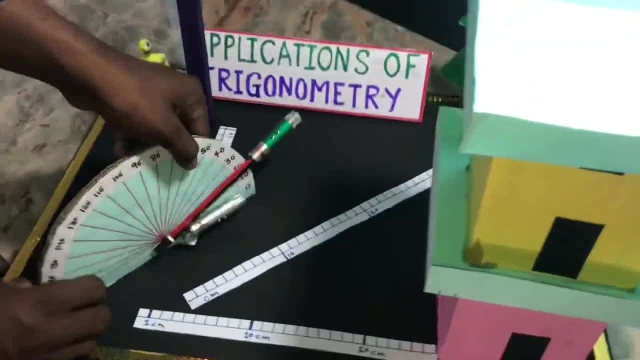 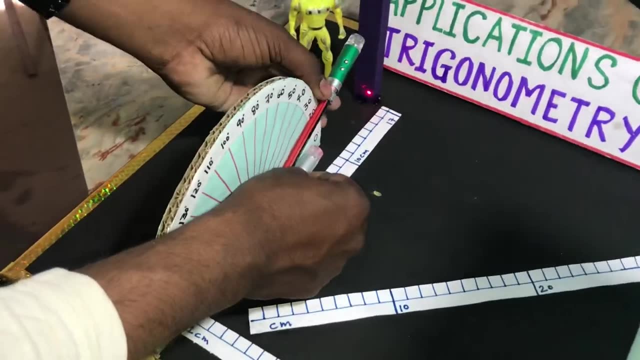 How will we find the height of the pole? So first we will find the height of the pole. So first we will rotate this clinometer. After that we will see from here. From here the angle will be measured, So from here you can see the laser light. 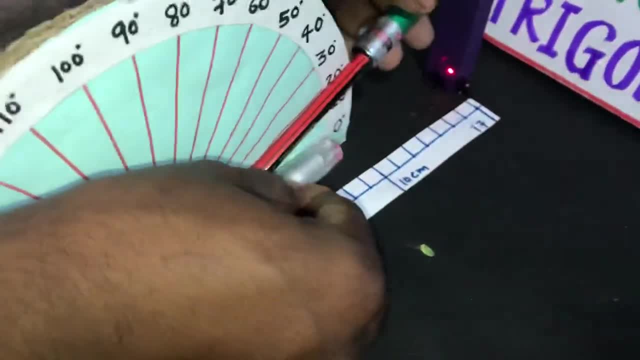 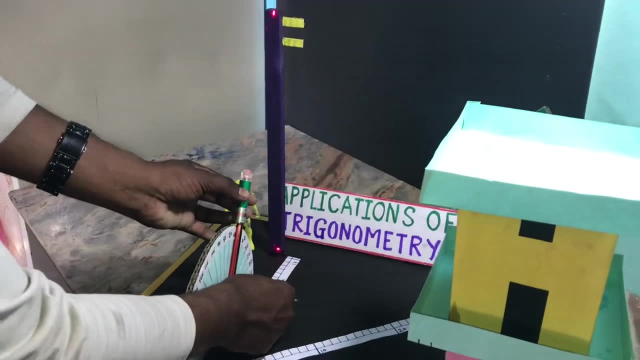 From here, So this is always 2 centimeters. There will be an error here And we are seeing how many degrees the angle is being made from here. So this angle is being made up to the pole: 60 degrees. The angle is being made up to 60 degrees. 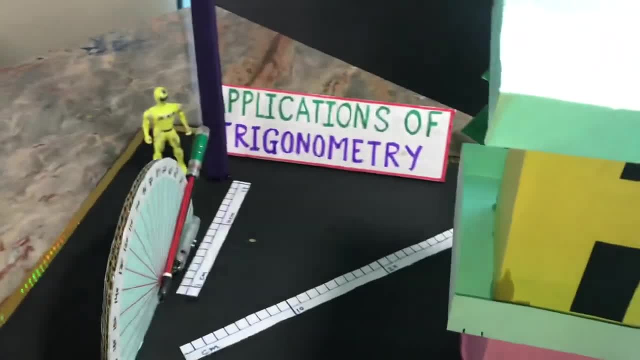 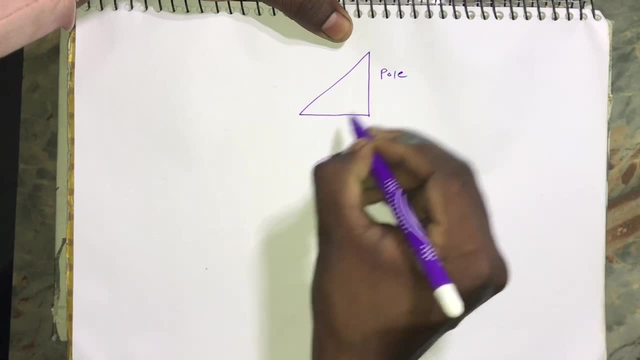 Ok, So we will apply the formula of 10.60 here, So we will know the height of the pole. We will find the height of the pole. This is the pole And this is the base. This is the hypotenuse. 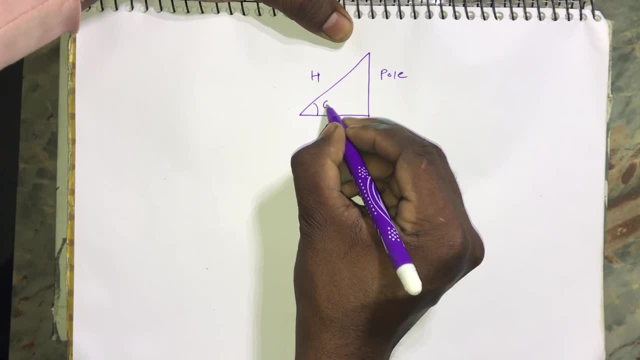 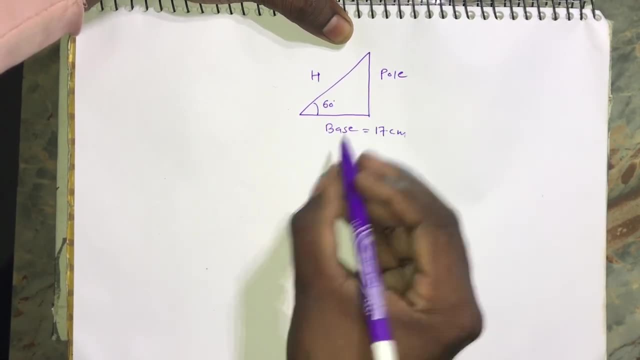 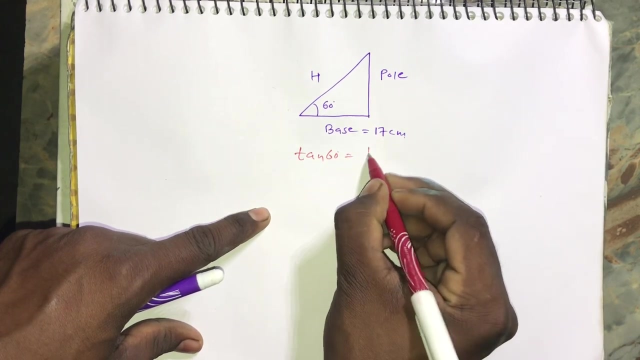 How much was this angle? 60 degrees. Ok, So we found the length of the base from the scale 17 centimeters. So we will find the length of the pole: 10.60 degrees is equal to perpendicular over base. 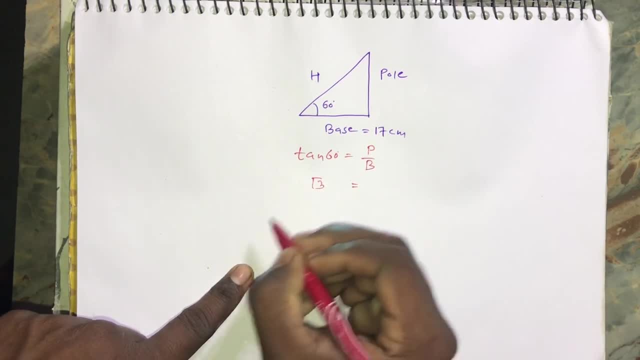 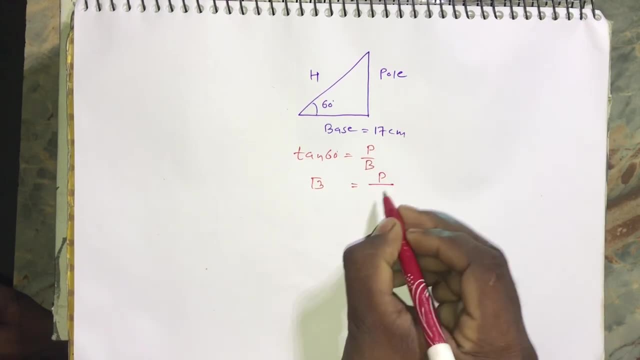 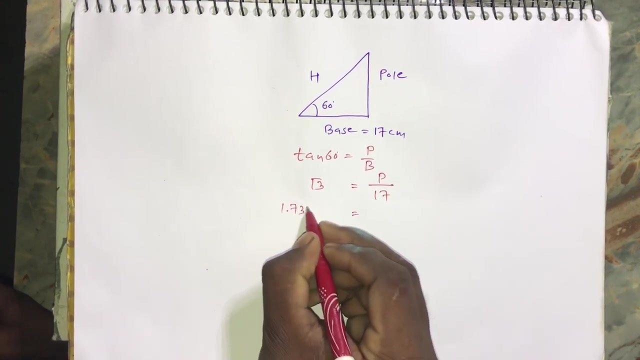 What is the value of 10.60? Root 3. And the perpendicular is unknown. And the base? What was the base? 17. So its value is 1.732 into 17 is equal to perpendicular, So the length of the pole is approximately 29 centimeters.